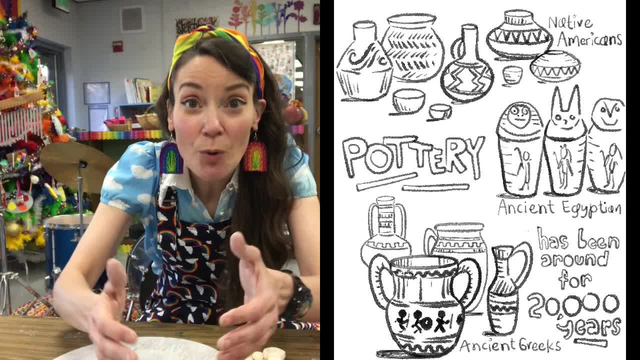 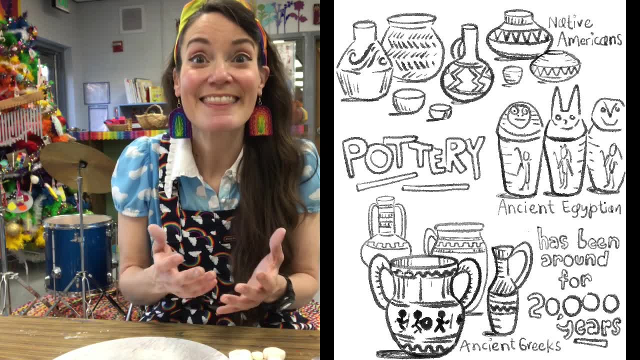 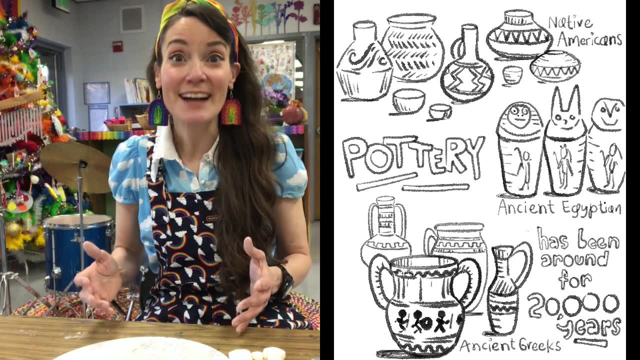 of time. Once they discovered that they could pull up something from the ground, mold it and shape it into clay and use it, then people were using it for all sorts of things, Not just for art, but for bowls and pots and cups. You can even still find some of these things If you're digging in the dirt. 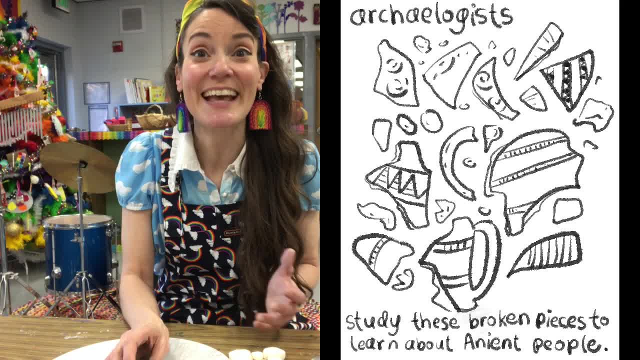 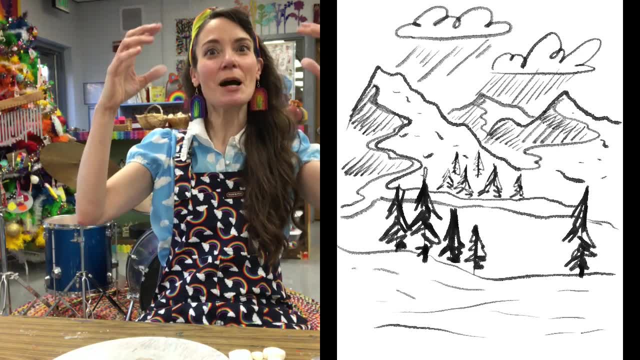 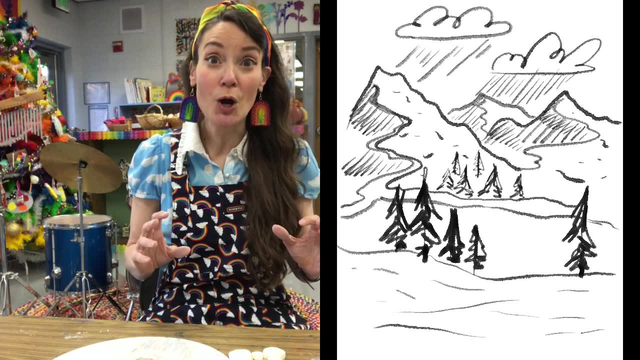 you might find some broken shards of old pottery and things made out of clay. Where did people, so long ago, get clay When it would rain? the rain would come down and it would start to wash rocks and minerals and different kinds of things Start to erode and fall down the mountain And as it eroded down the mountain, it picked up a. 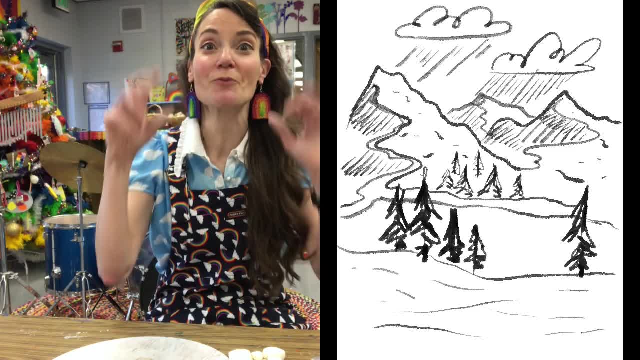 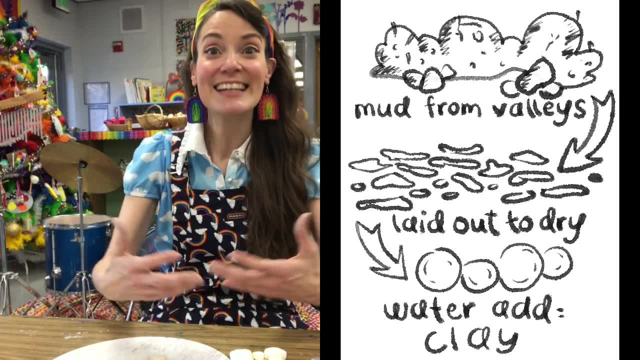 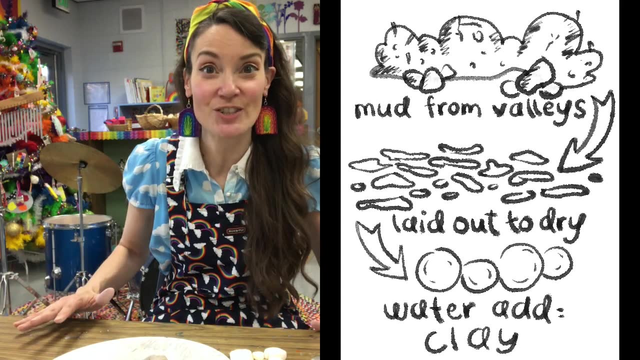 little bit of speed and grabbed more rocks and more minerals before landing at the bottom of the mountain. When it did, Native Americans would collect that clay, take it home with them and then lay all that clay out on a table outside in the sunshine to dry. Why would they want their? 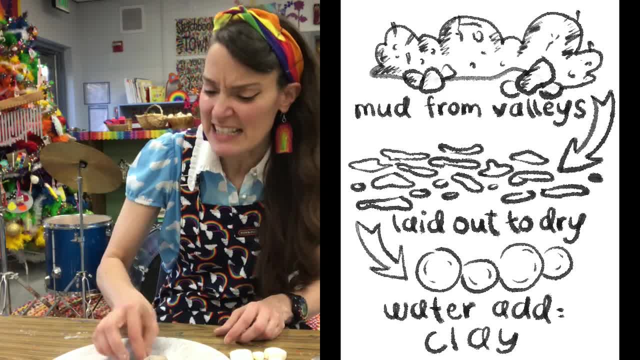 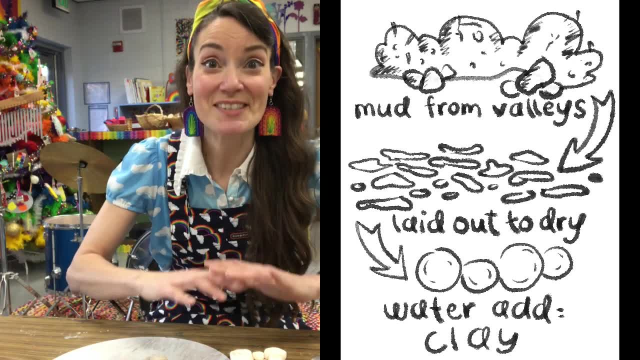 clay to dry. Well, because some of that clay might have had sticks Or twigs or rocks that were just too big, and they would have to pluck and pick those out. Once they were finished with that, they were left with a beautiful fine powder, for which they added: 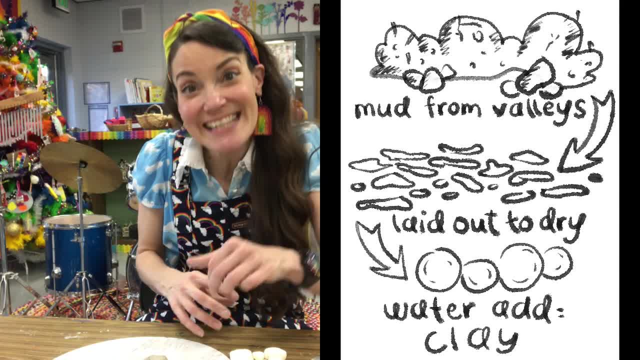 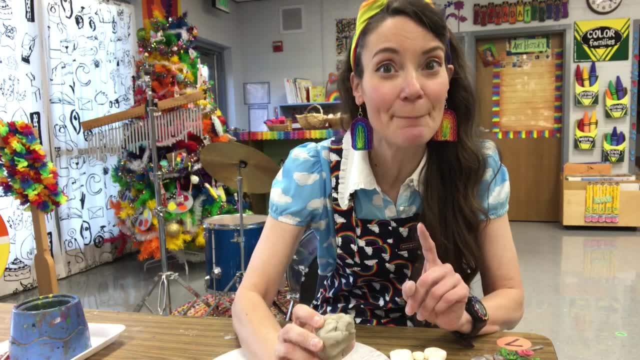 more water back to, and then they squished it all together, making their clay. The clay that I purchased for you is made in a similar way, but in a factory, So on a much bigger scale, but it's still dirt from the earth. 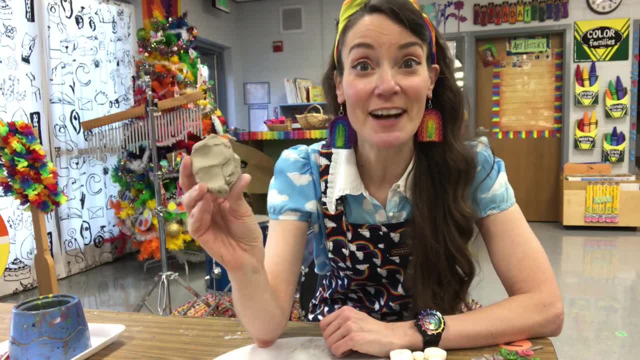 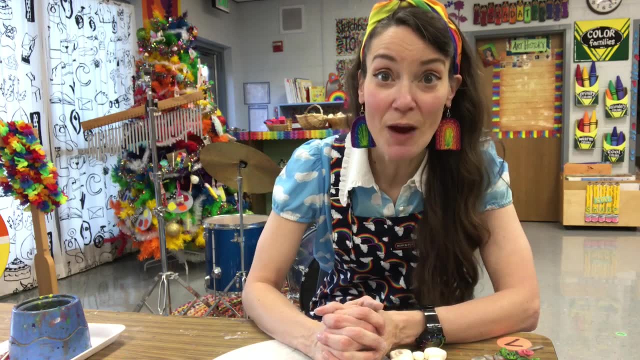 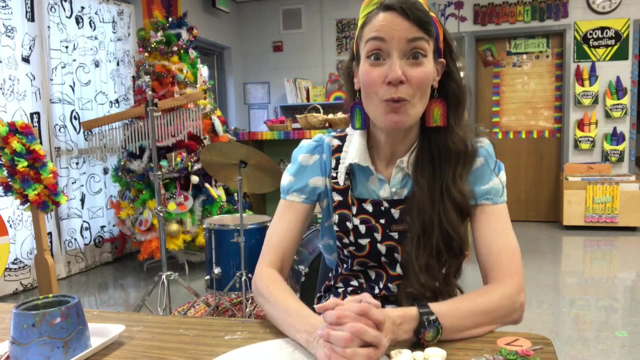 Clay, because it's dirt from the earth, comes in a bunch of different colors. Once you're finished with your clay piece, then we want our clay piece to dry, That's right. we don't want it to stay soft and squishy forever, because we want to be able to keep it forever, Your clay, when it's. 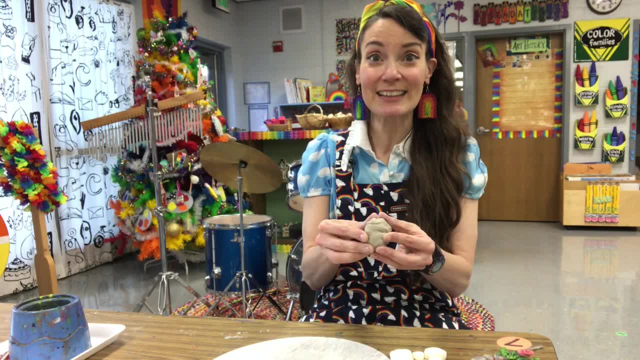 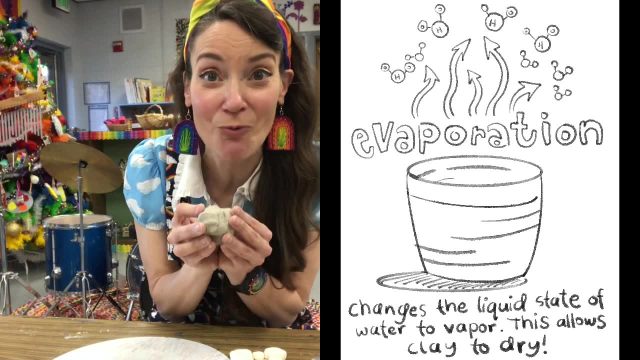 drying, we're allowing the water that's in the clay to evaporate or leave the clay. There's tiny little cutesy-rootsy molecules of water inside this clay and they're going to evaporate. So when we're finished with our clay, we want them to go away when we're finished with our piece. so 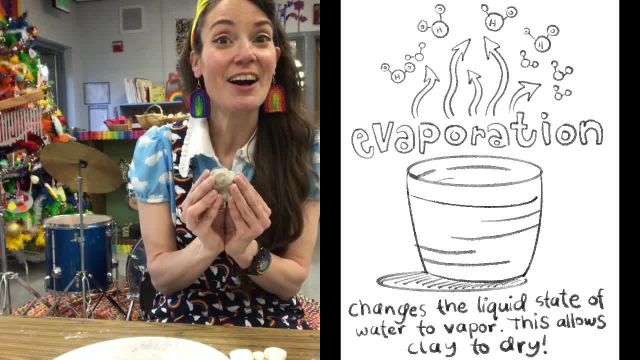 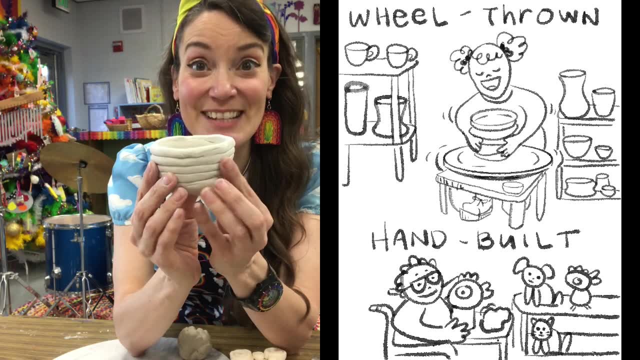 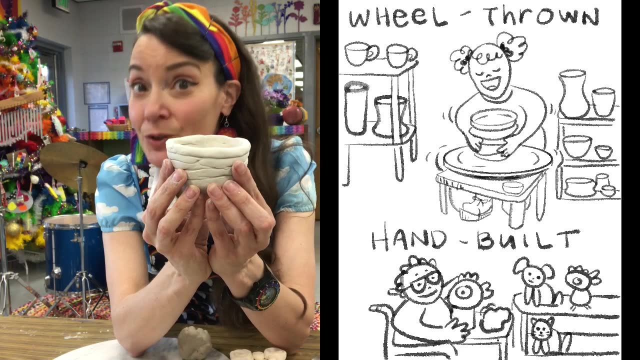 that we can move on to the next step of firing our piece in the kiln. Here's a little bowl that I made by hand. When you make something by hand, it's called handmade. When you make something on what's called a potter's wheel, that's called wheel thrown. And here we're going to be building. 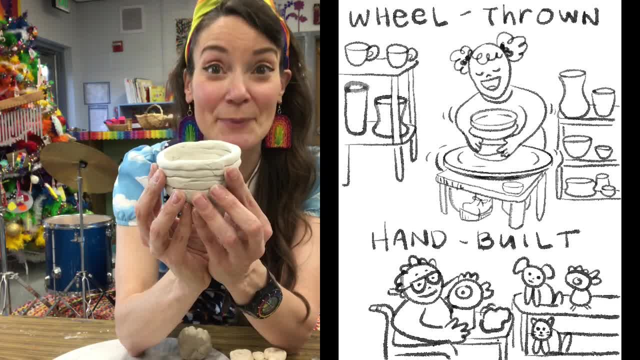 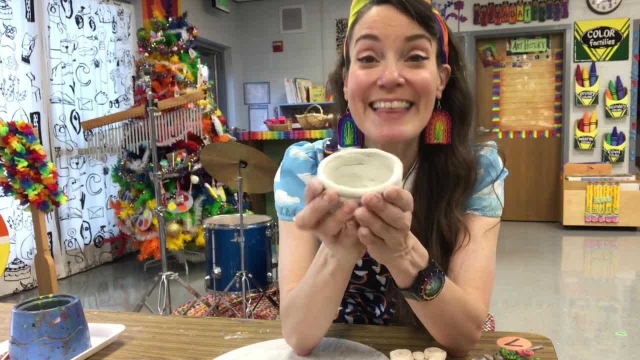 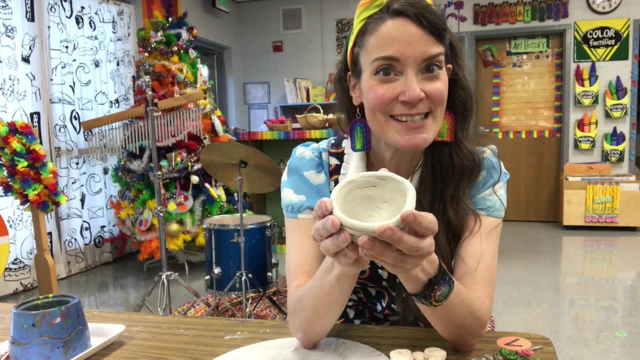 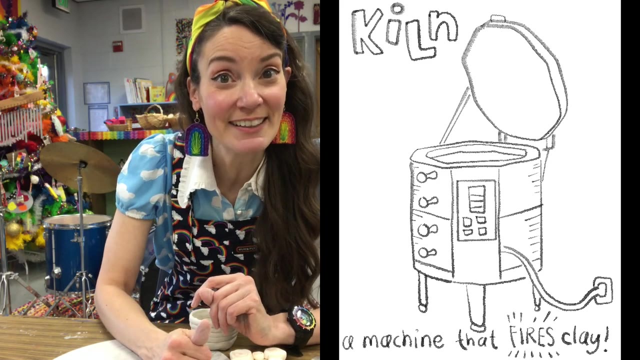 everything by hand, so everything we create will be hand-built. When your clay piece has been completely dried and there's no squishiness to it, this is what's called bone dry. It's as dry as a bone. It's now ready to go in something called a kiln. What is a kiln? A kiln is an oven, that's. 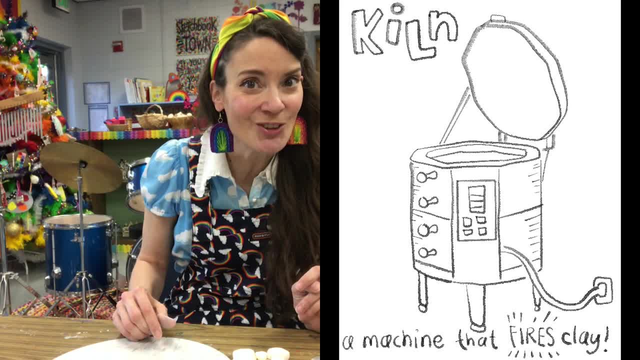 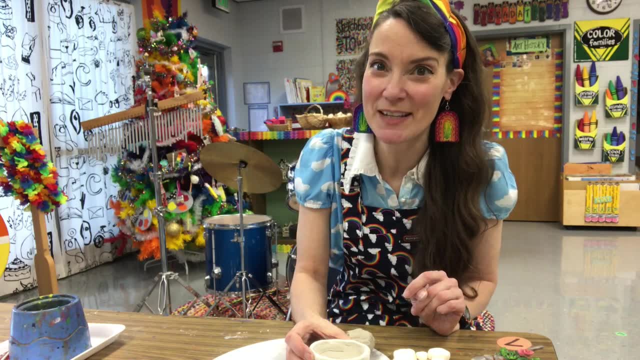 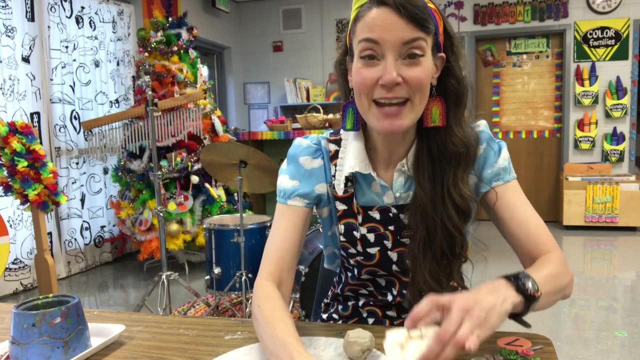 made specifically for clay. A kiln's highest temperature is 2,000 degrees. It can reach that high temperature to get your piece dry. When it comes out of the kiln it goes from this gray look to this bright white look- A clay piece. 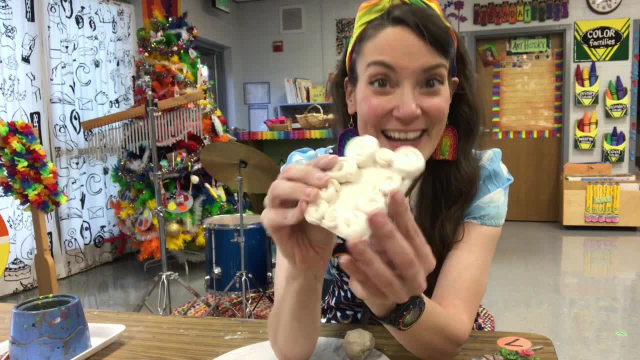 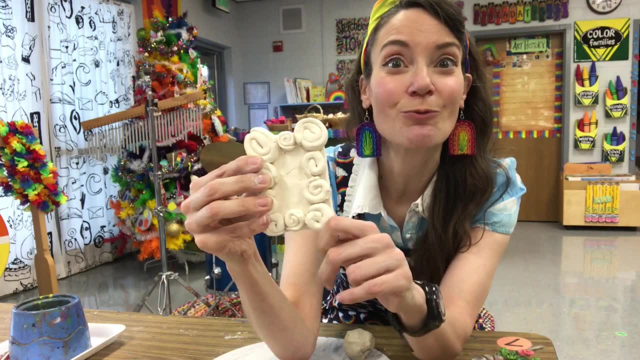 that's fresh out of the kiln is called bisque, Or, if you're from England, it's called biscuit wear, which just means the same thing: Nice and hard and ready for you to keep or paint. You now get to add. 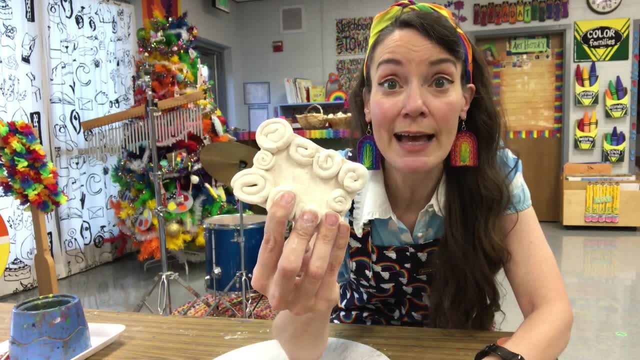 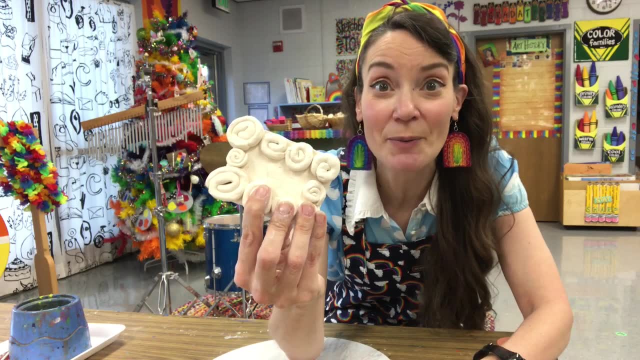 the color, baby color. Now, when it comes to clay, you could approach adding a little bit of color the same way you do a piece of paper. You could use paint, You could even use markers, crayons and oil pastels, Or you could do something that traditional clay artists use. 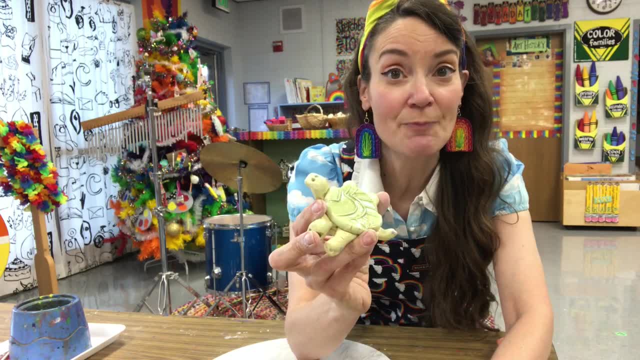 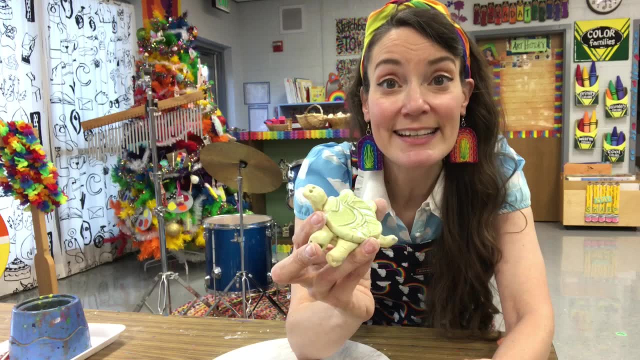 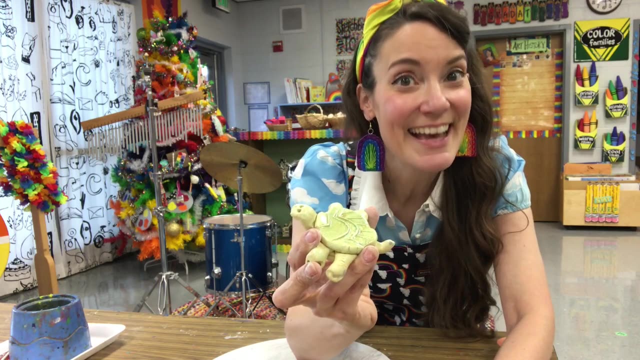 which is called glaze. Glaze is a special kind of paint that is just for clay that has very small, sometimes big pieces of glass in it, And when you cover it with glass it definitely doesn't look like much because it has to go in the kiln again The second time it's in the kiln. 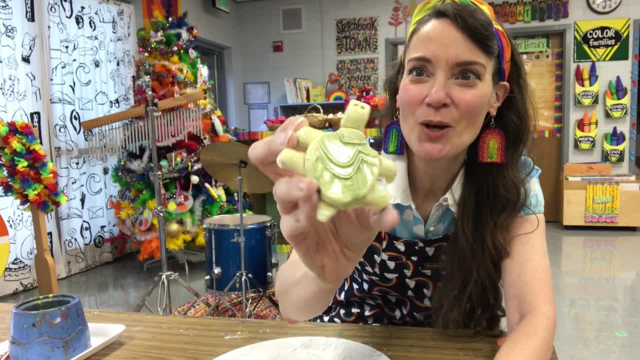 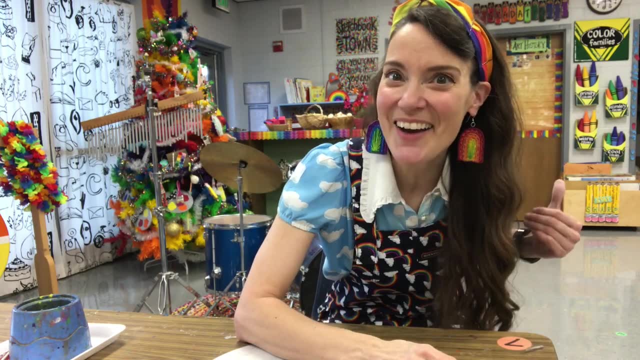 those little pieces of glass melt and they come out really shiny, just like this. What's that? You want to see what my kiln looks like? Well, let's go, I'll show you in the kiln room. All right, guys, this is the kiln room. It's called the kiln room because guess what's in here.